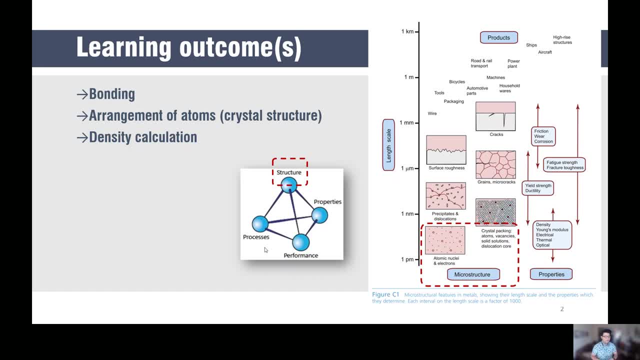 So let's just begin the journey. The learning objective today is going to be Bonding, arrangement of atoms, crystal structures, and by the end of this lecture series on this chapter, you will learn how to calculate density, which is a material property for different types of material with different types of crystal structures. 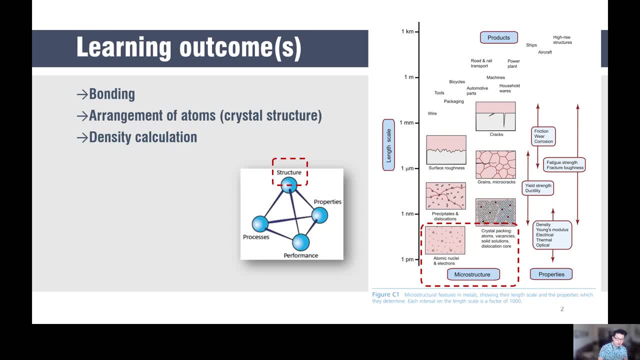 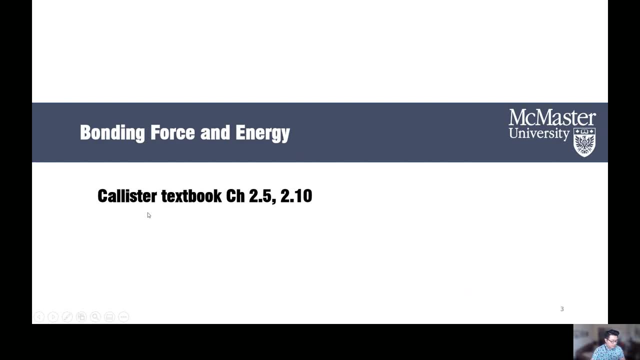 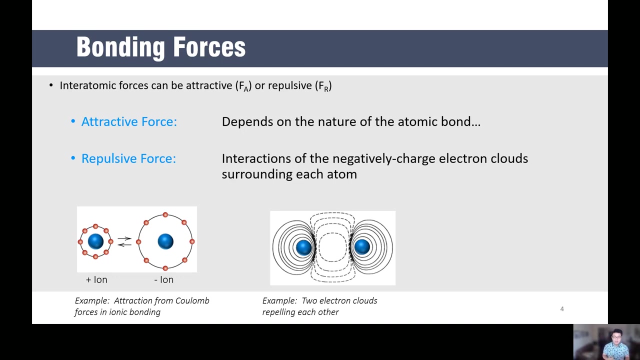 So we're now really going into talking about the fundamentals of how atoms are being bound together and arranging each other. Okay, So let's start with bond force and energy- chapter 2.5 and 2.10.. So there are many types of bonds. You may have already learned from your chemistry or physics class that there are ionic bonds, covalent bonds. there are secondary bonds, such as hydrogen and van der Waals force. 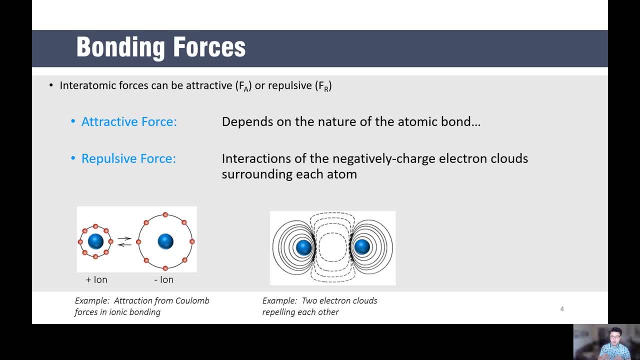 You have also learned that maybe there's metallic bonds. So in the chapter there's more details about that, And here we want to illustrate And very important concept, which is the differences between attractive force and repulsive force. So let's pick an example. 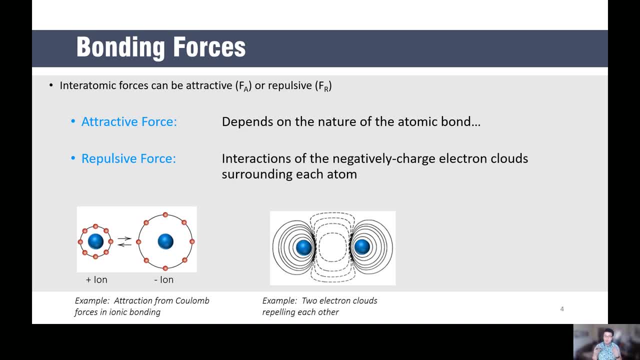 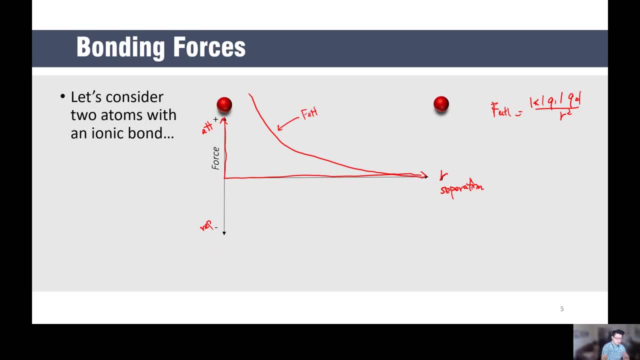 And you may have already learned attraction because we have looked into our physics class, And you may have already learned attraction because we have looked into our physics class. What happened? if so- this is, by the way, this is Q1 and this is Q2, let's say: 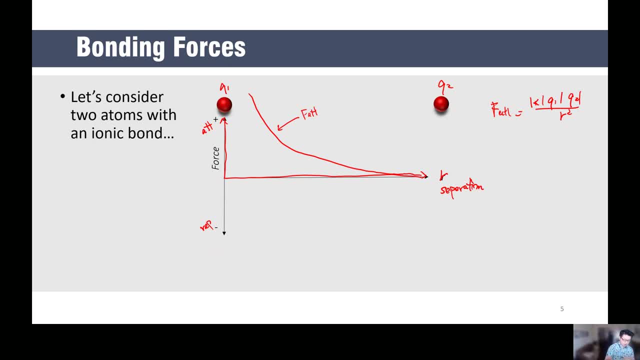 So what happened? if you have a separation that are getting very close, then there's a repulsion force And the repulsion force. you may not have learned that yet in the in the physics class, but that's okay. um, for now we just think of it as a short range, or the force, and it will arise much. 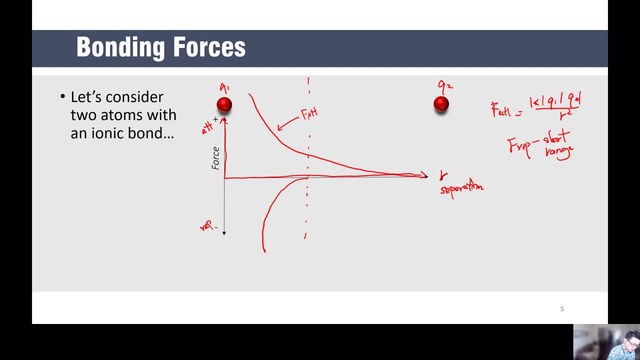 when r is at a much lower distance, but then it would. suddenly this repulsive force will increase very drastically as distance becomes closer to zero. so this is the repulsive force, and in your physics class you may have learned that how we can measure the equilibrium is through a summation force of, so the net force. 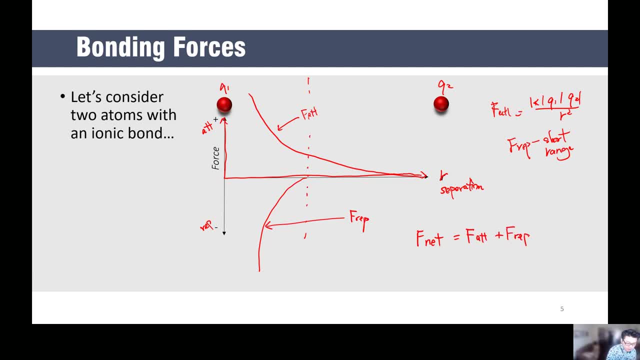 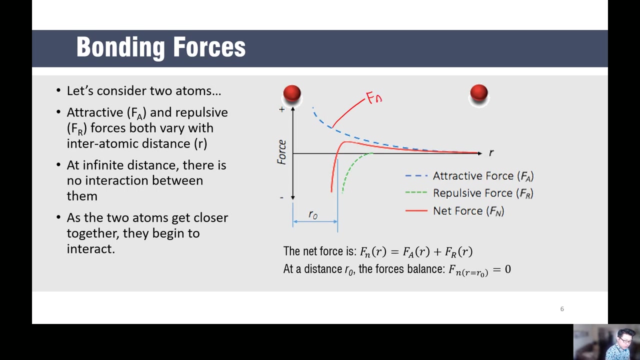 of attraction plus the repulsion. it's in the attraction and repulsion of opposite. there's a particular point at which the force abounds altogether and there's a equilibrium point where the net force is equal to zero. so let's see how that works. so here the blue curve is the attraction. 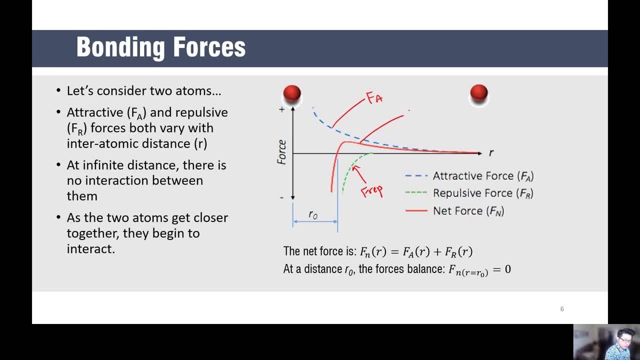 and the green curve is the repulsion, the red curve is the net force. if you add the positive, so if you add the net attraction and the repulsion, you'll find that the red curve will, at the very long distance, will look identical to the attraction force and then 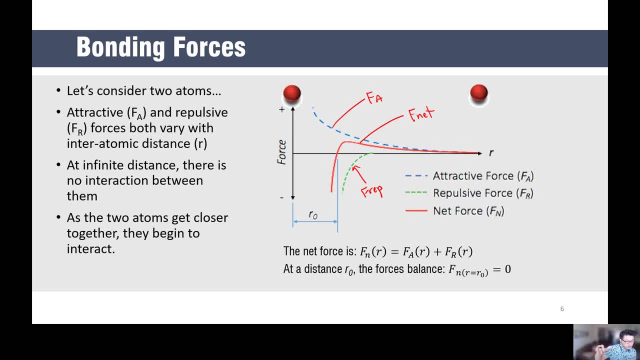 it will curl in, but then, because of short range repulsion is coming in. eventually it will drop back down and at very low distance it will look almost like the repulsion force, this particular point at which that the positive, the attraction and the repulsion are canceling. 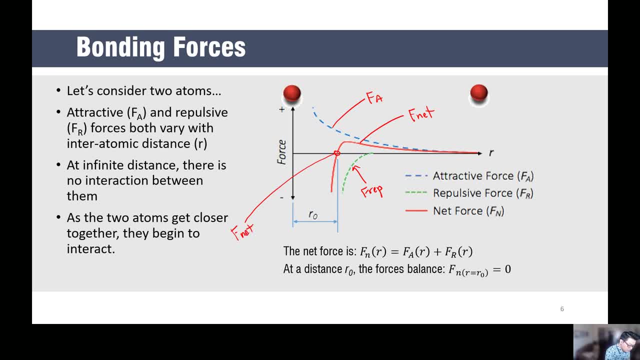 each other, we have a net force of zero, And this is important. This basically saying that if you look back in the whole picture, you have two atoms. they have different charge and that's why they're forming ionic bonds, And basically what bonds is is the balance between the attraction and repulsion, And so 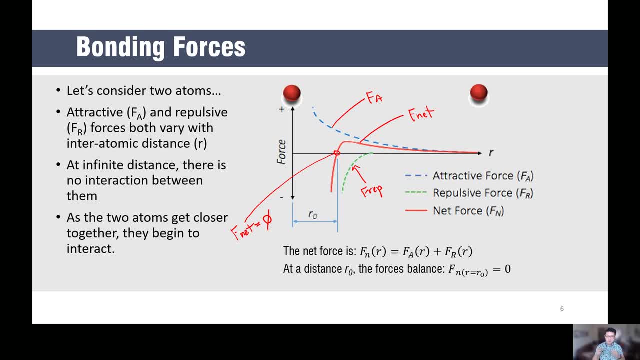 an analogy to this, you can think about a spring. When I pull a spring, it wants to bounce back. When I push the spring, you want to push away. Here is very similar. In a spring system, the attraction and the repulsion are identical, But in this particular case the repulsion. 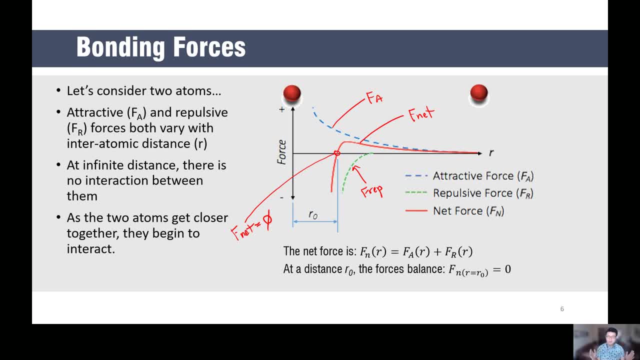 the attraction and the repulsion have different range order, leading to the case where we have this funny net force curve. But there's still an equilibrium point, just like the spring. If you leave it alone, it will have an equilibrium distance in this point. 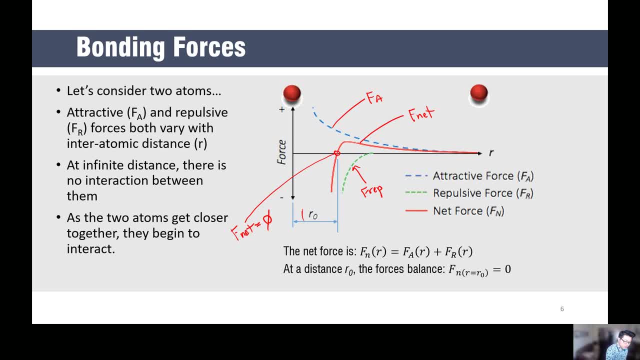 case, we have an equilibrium distance, which is our norm, And this equilibrium point is important. This is what atoms like to stay at for a particular temperature, And so this is the atomic separation, And if we understand atomic separation, we can then start to think how atoms are put together. 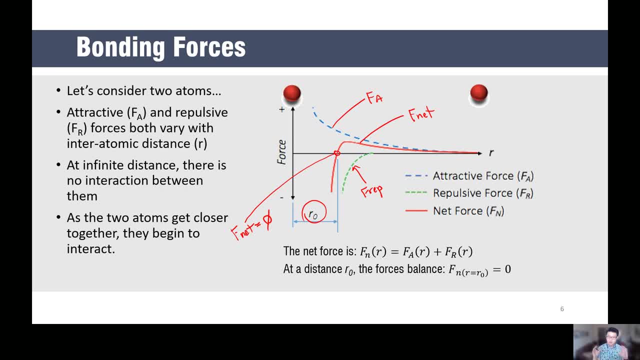 So let's give you an example. Let's say if I have some kind of crystal that is being grown, Let's say I am creating a salt crystal and I want to find out the density of the salt crystal. So it may go from the molten state and then, when it cools down, it will form this kind of 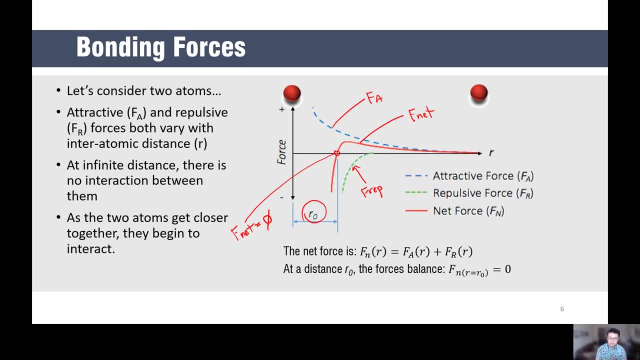 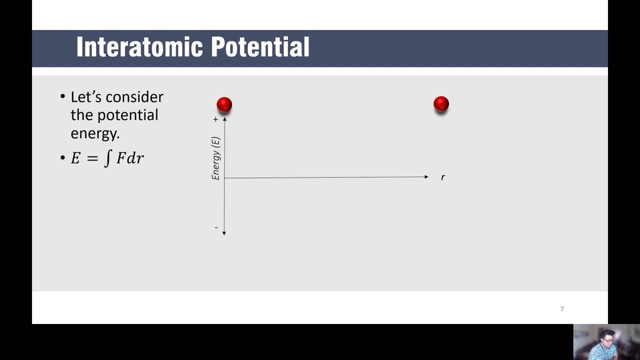 crystal, salt crystal, in which you can find that the atoms, each of them, have an equilibrium, atomic separation. And if you know that atomic separation and you know how these atoms are arranged together, then you can start to calculate the density. So the same plot of the force curve can be also represented by the energy curve. 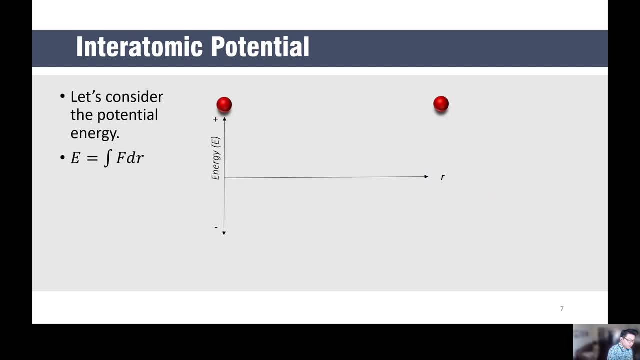 And here is the potential energy curve. And so one thing that you need to know is that energy is equal to the integration of force with respect to dr, Or another way of talking about that is: force is the derivative of e with respect to r. 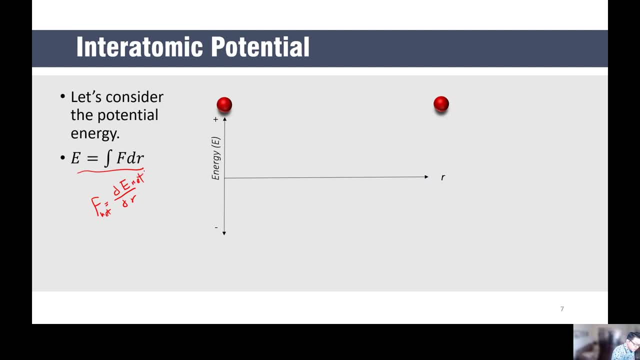 And this is net force and that e. So we can. we write this curve in terms of energy instead of force. So the attraction is k, q1, q2, a plus uno square, And, And the energy of attraction is going to be integration of f. attractive dr. 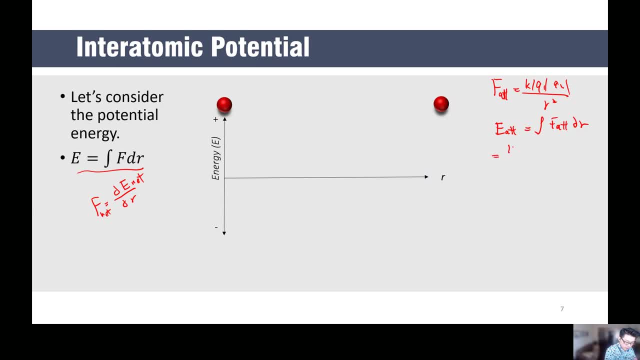 And we can write this as k, q1, q2 over r, with a negative sign here. Okay, so this is important, because what we're saying is that if you have an attractive force, the energy is negative. If you have a repulsive force, the energy in this scale is positive. 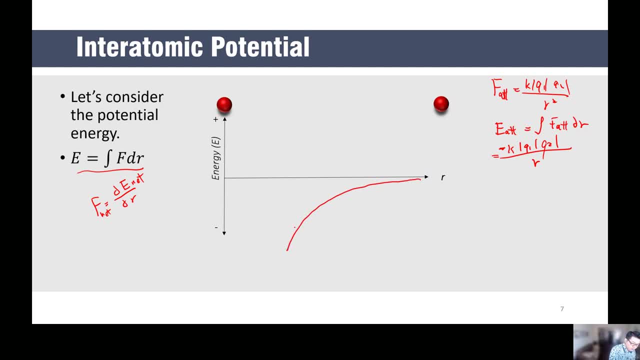 So we can redraw this graph And this is the long range of order, And so this is the attraction energy, And similar argument at short range will have a repulsion energy. This is the repulsion energy, Okay, And with this we can start thinking about the net energy. 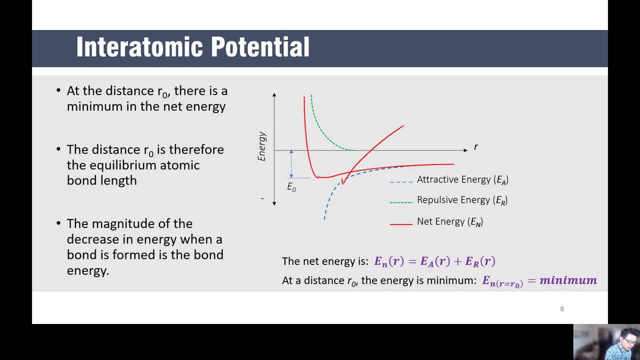 And the energy looks like this. So the attraction force is the blue curve And the repulsion curve is the green curve And the net is the red curve And you see the red curve here on the left The red curve is the same. 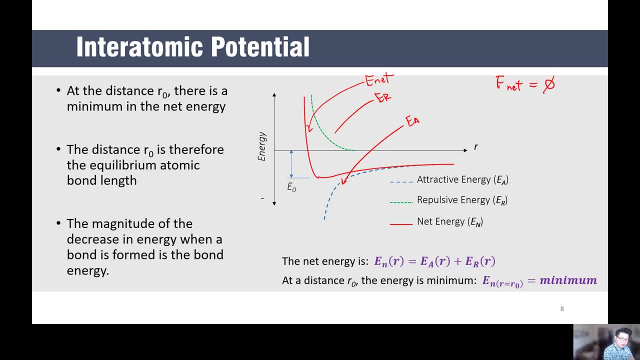 The red curve is the red curve on the right And the red curve is the red curve on the left. The red curve on the left is the direct current output, And we can see here that we have these twoας the same energy. 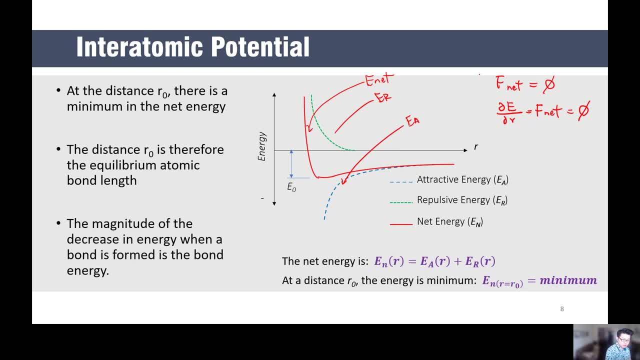 So we're able to write known energy. What's going to happen next? What's going to happen? Okay, what this statement is referring to is this magical point where the energy is at the minimum, And so this is R0, the same R0 that we see from the previous curve. 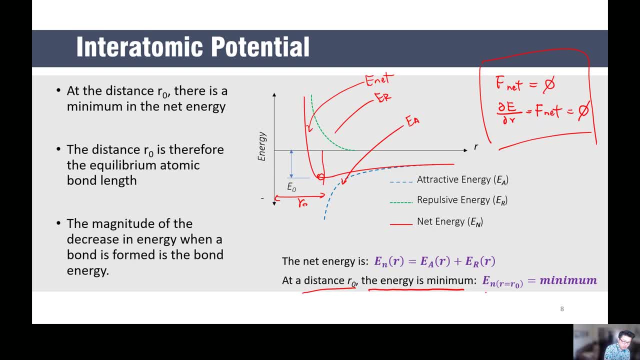 So at R0, the energy is at the minimum. So this is the same thing, but now we're talking from a thermodynamic point of view. We're saying that the two atoms would like to stay at a distance of R0, because at this particular distance the energy of the system is at the lowest possible. 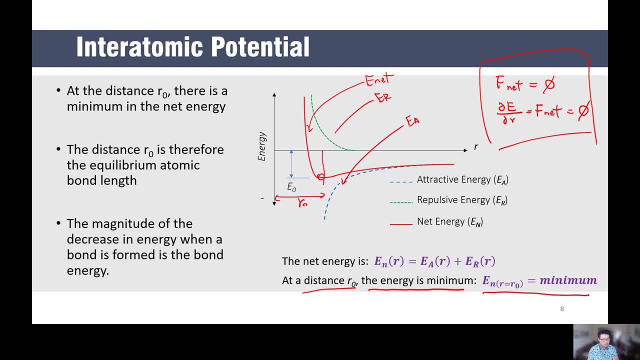 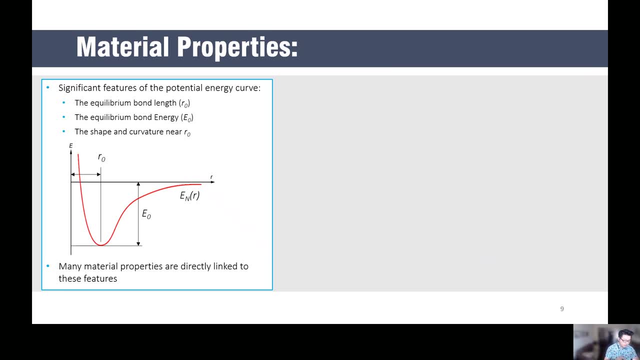 So what's so cool about this is that you can start to infer some kind of material property by looking at the atomic separation as well as the energy scale of this curve. So one thing that you might ask is: OK, How much energy do I need to break this particular bond? 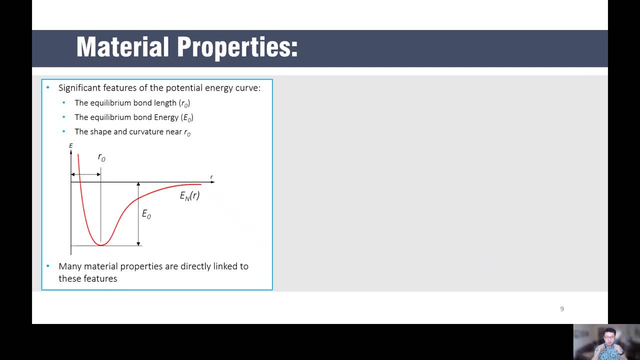 So these two atoms are really attracted to each other, but then at a short range they repair each other, So they sit in this particular distance. How much energy do I need to pull it in order to break it? If I pull this, then the energy I need to subscribe is basically the distance from the minimum point to the x-axis. 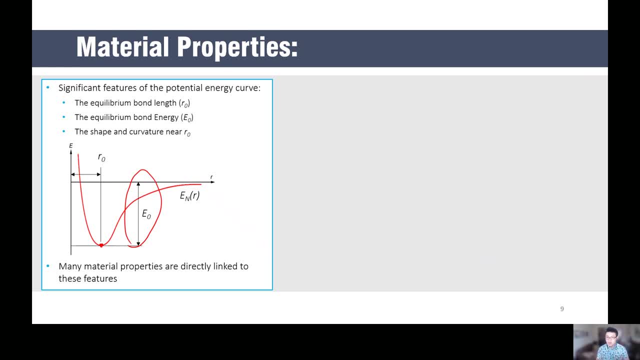 So this is E0.. So this is the bond energy of a two atom system, And so one thing that can infer from this plot is melting point, for example. So in this particular system, bond one has a deeper minimum point And bond two has a shallow minimum point. And bond two has a shallow minimum point And bond two has a shallow minimum point, And so what it's saying is that bond one, the two atoms, are actually bonded together stronger with a stronger energy, which means if I want to break the bonds, I need to subscribe more energy to break them. And so what it's saying is that bond one- the two atoms are actually bonded together stronger with a stronger energy, which means if I want to break the bonds, I need to subscribe more energy to break them. And so what it's saying is that bond one- the two atoms are actually bonded together stronger with a stronger energy, which means if I want to break the bonds, I need to subscribe more energy to break them.